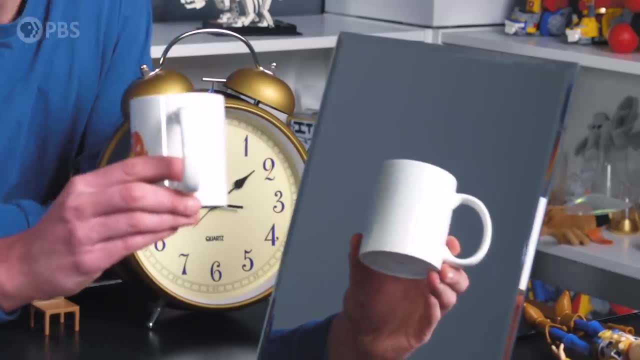 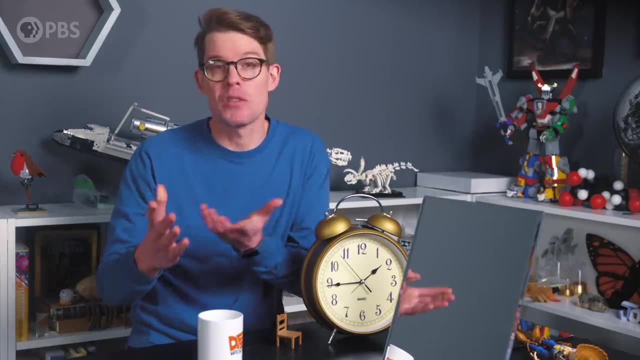 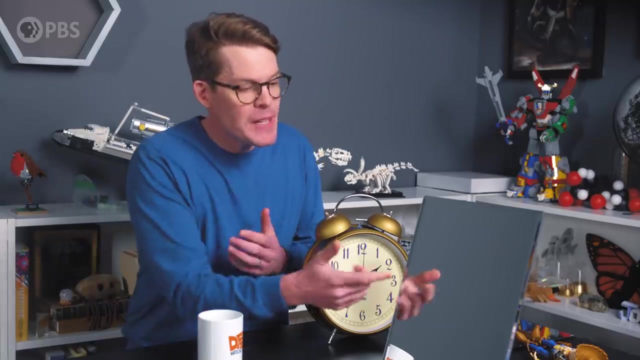 And well, take this cup. It looks like a normal cup, Except that the writing on the cup is reversed. So maybe mirrors only do their reversal magic on words and numbers and not furniture. That doesn't make any sense. I mean, the left and right side of this mirror are the same as the top and bottom. 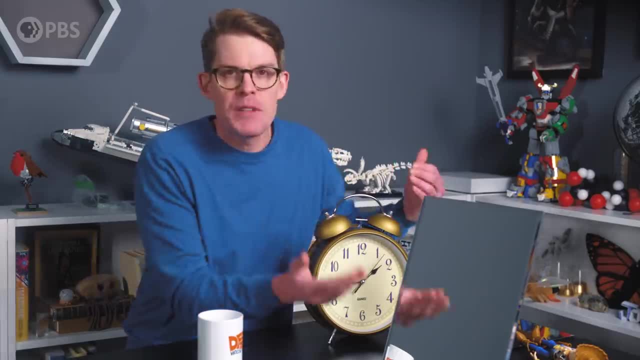 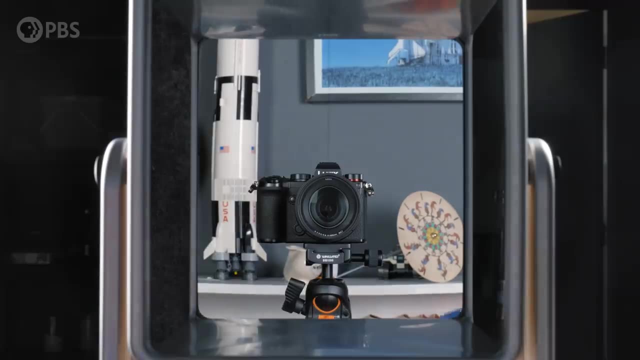 They're similar, They're smooth, They're shiny. Why are only the left and right flipped? Why isn't my head on the bottom and my feet on top, like they are in this mirror? And why does this mirror not reverse left and right? 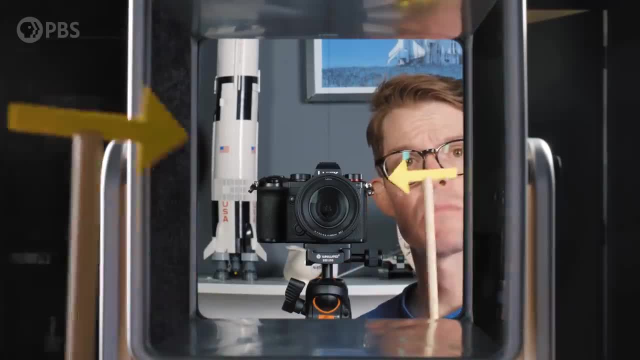 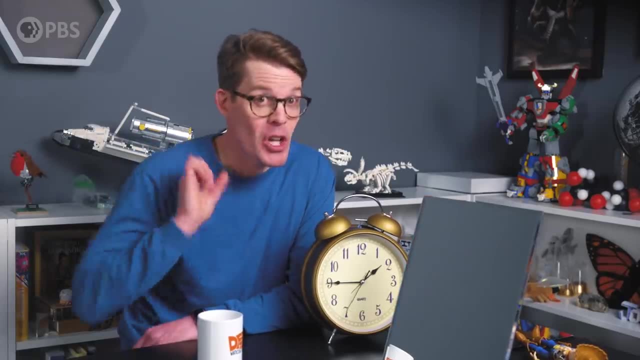 My left hand is the left hand of my reflection And right points to his right. Mirrors are weird And it's about time you learned how they really work To really understand the magic of a mirror. it might help to leave our three-dimensional world behind. 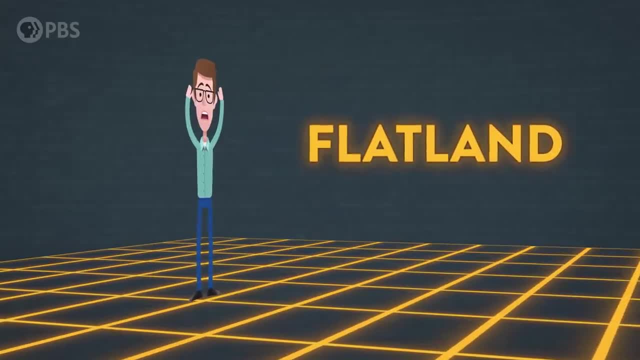 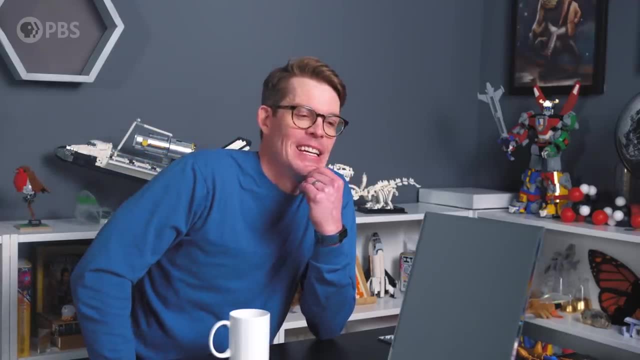 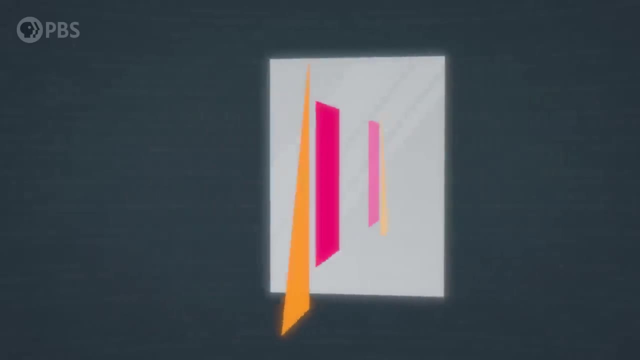 So we can grab a few eyes for a second and enter Flatland, a world inhabited only by flat two-dimensional characters. It's a pretty plain existence. Let's move on. Meet Mr Triangle and Miss Square. When they look in the mirror, each of them just sees a line. 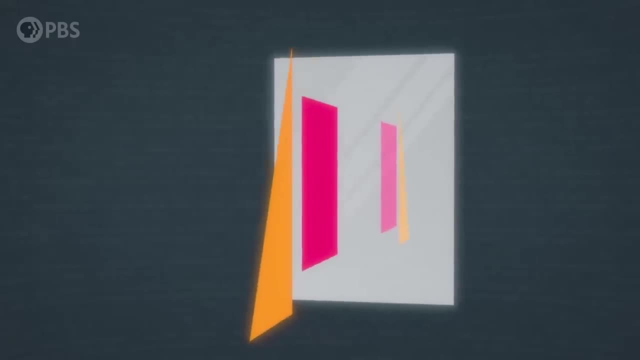 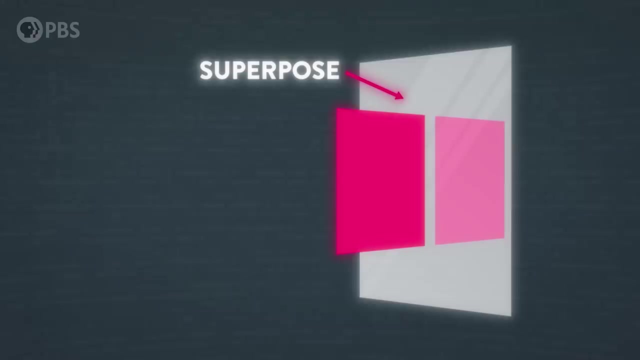 But from our three-dimensional point of view we can see their whole reflection. If we imagine sliding Miss Square into the mirror, she can cover—or superpose— reflection point for point without turning her around. In other words, she's symmetric. 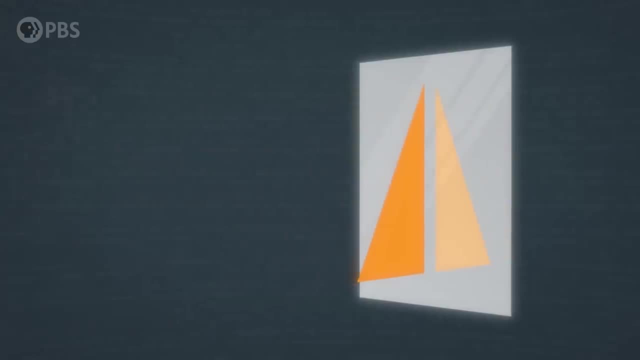 But if we imagine sliding Mr Triangle into the mirror, there's no way he can cover his mirror image without us rotating him in a higher dimension, Which would be a very strange experience for him. Mr Triangle is asymmetric. He can't be superposed on his reflection. 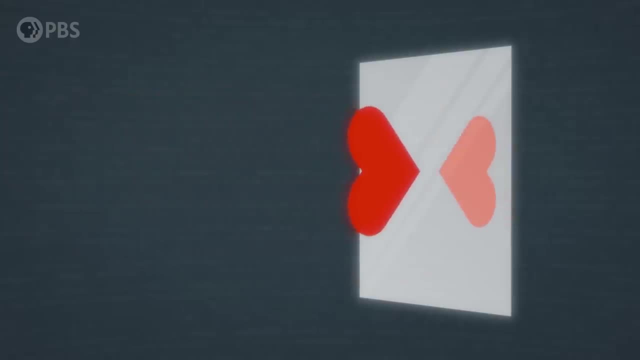 In Flatland. a heart is asymmetric if it approaches the mirror like this, But it's symmetric if it looks in the mirror like this. It has an axis of symmetry running up and down a line that divides it in half, and if you put the edge of a mirror along this axis, you get the original shape. 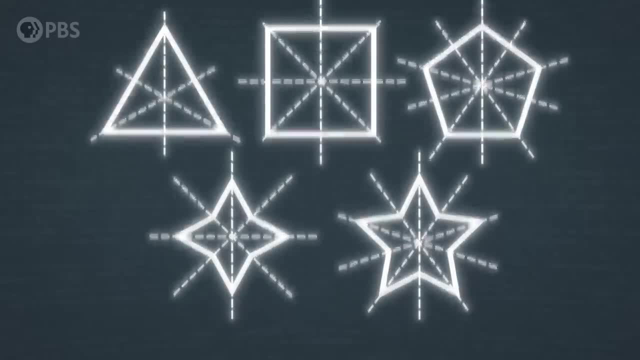 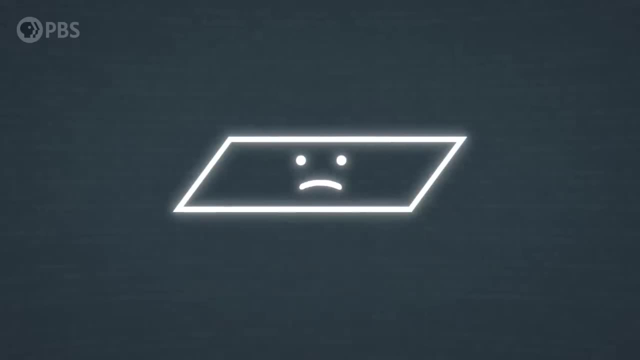 Different shapes in Flatland have different numbers of axes of symmetry. A circle actually has infinite axes of symmetry, Except poor Mr Parallelogram. No axis for you. you're just as asymmetric as they come. So we've been playing around in this imaginary two-dimensional land. 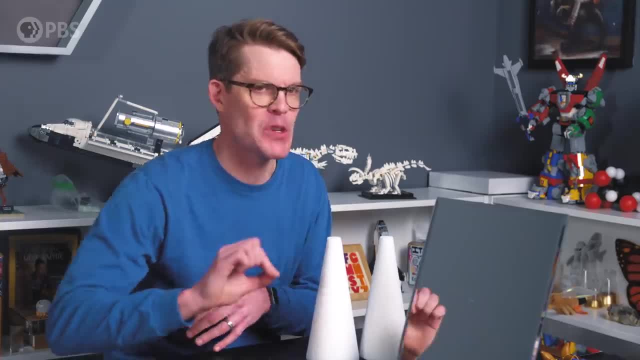 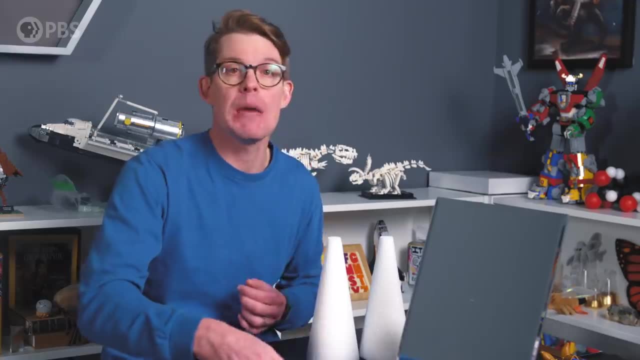 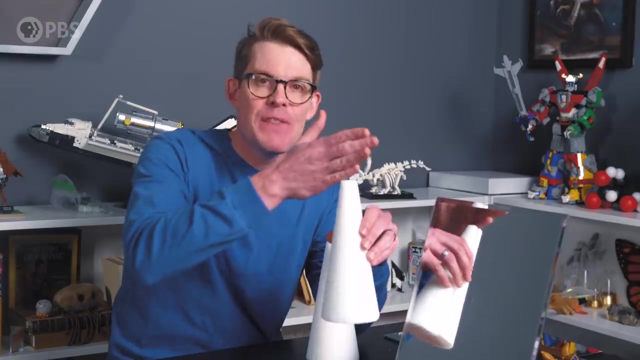 To hopefully give you a hint about what it is that mirrors really do. So just like 2D shapes can have a 1D line of symmetry, 3D shapes can have a 2D plane of symmetry. Take this cone: It actually has infinite planes of symmetry rotating around its center. here. 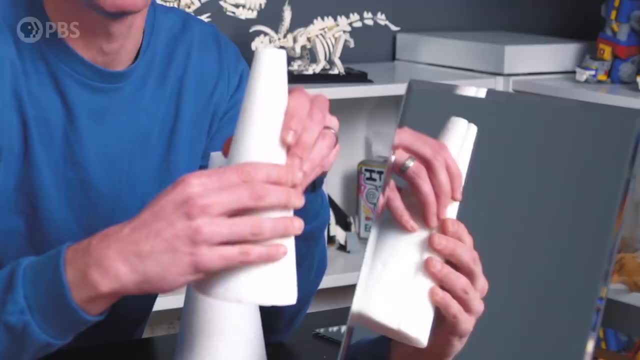 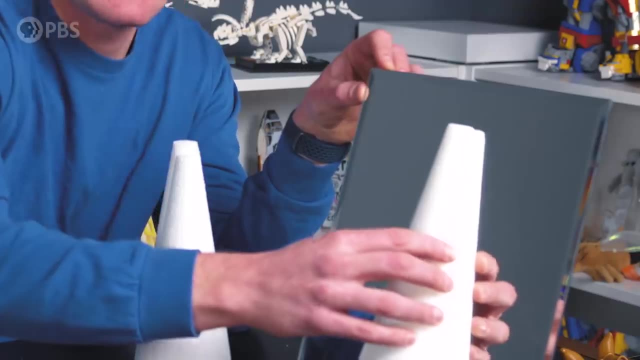 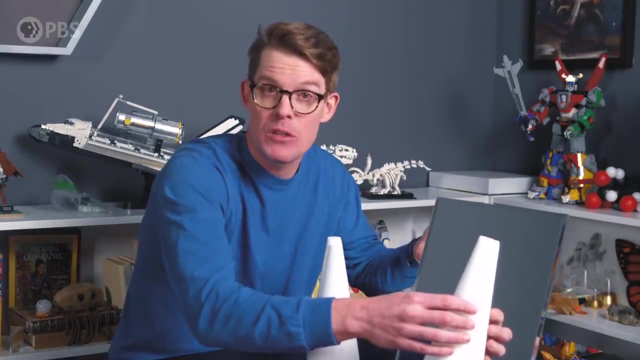 And if we slice along one of those, we get two half-cones. Each of them completes the other. It's as if we split it into the mirror and it overlaps with itself. This happens because the mirror is parallel with the plane of symmetry. 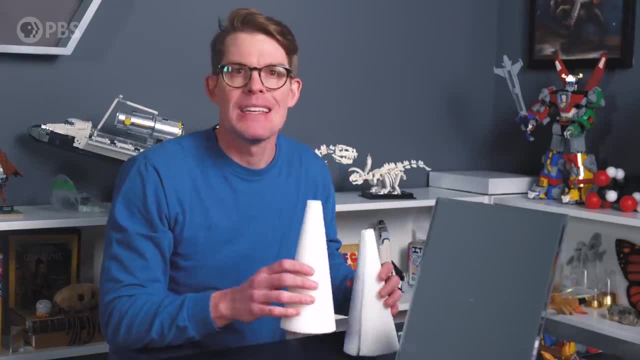 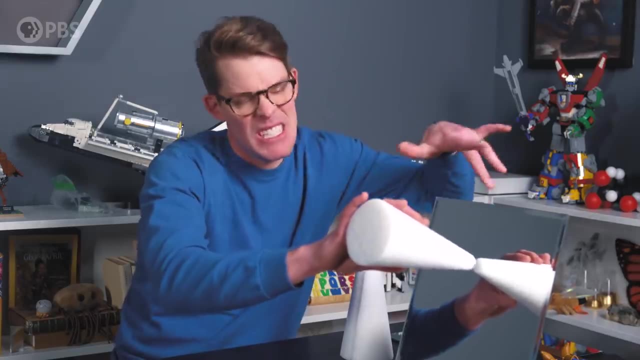 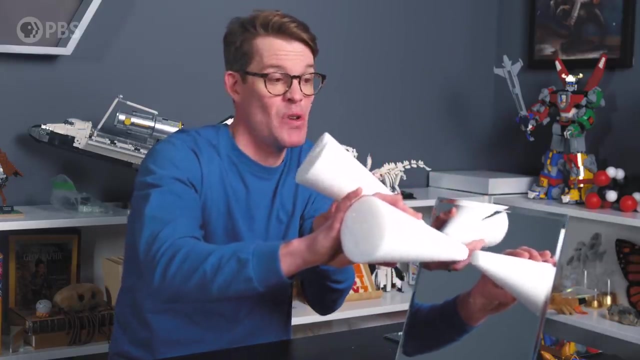 But what if we point the cone so that the mirror is now at a right angle to the plane of symmetry? Suddenly, what we see in the mirror doesn't really line up anymore. It's been reversed. Now we could imagine rotating this cone into the mirror. 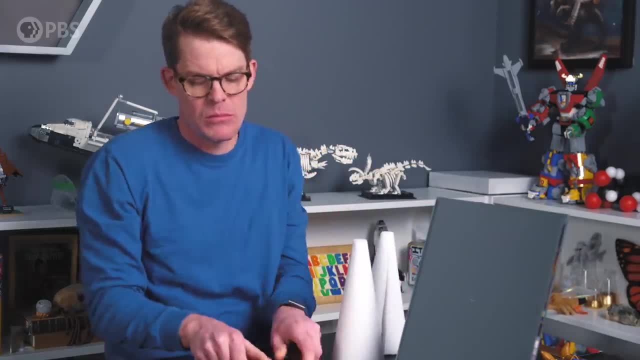 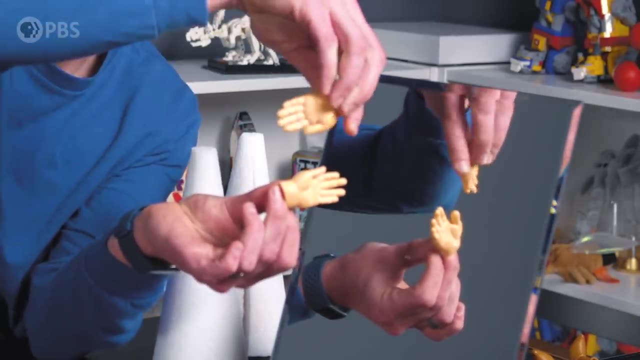 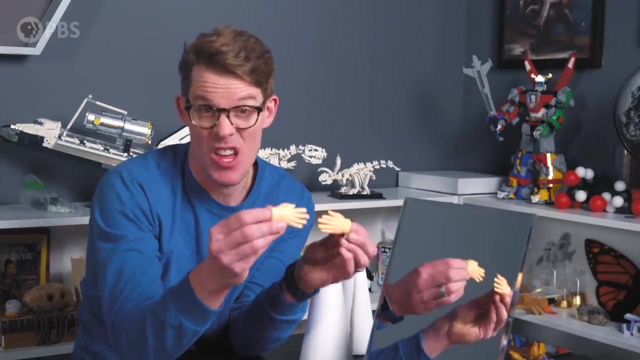 So that its point was facing out. But what about these? There's no way to rotate a hand around so that it neatly, totally lines up with its reflection. Shapes like these that are the mirror image of each other, but they can't be superposed. 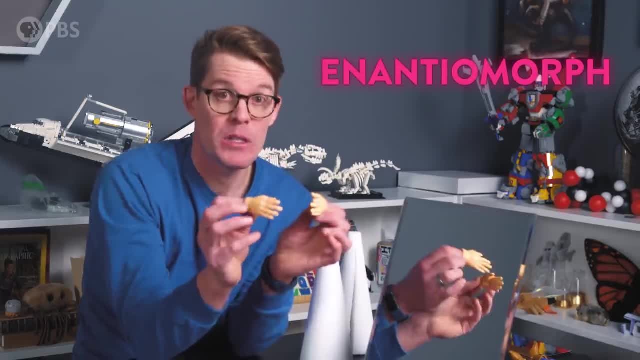 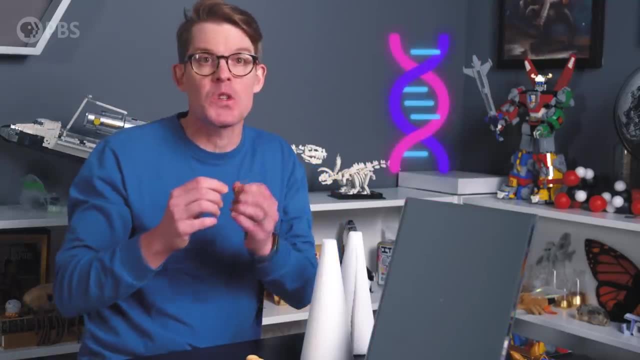 on each other. they're called enantiomorphs, Which is a cool word. Left and right shoes are enantiomorphs, So are your ears, Or a helix, or spring that curls right and another that curls left? Same but different. 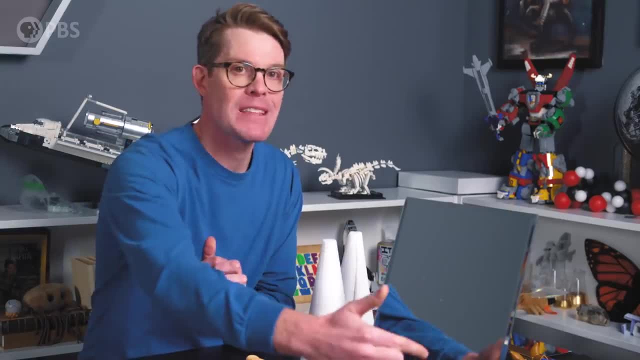 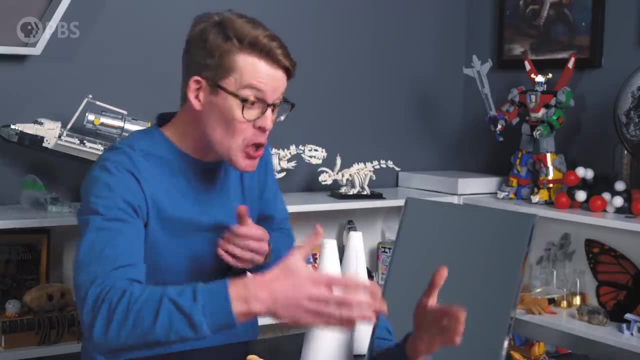 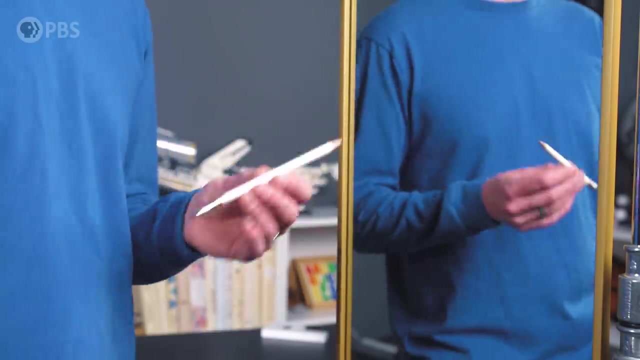 And this is why mirrors seem to reverse left and right, Because they actually don't reverse left and right. They reverse forward and back. You are looking at your enantiomorphic self. To make this forward-backward reversal more clear, take a look at this pencil. 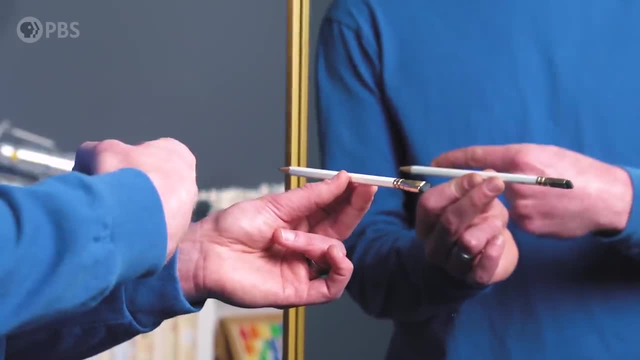 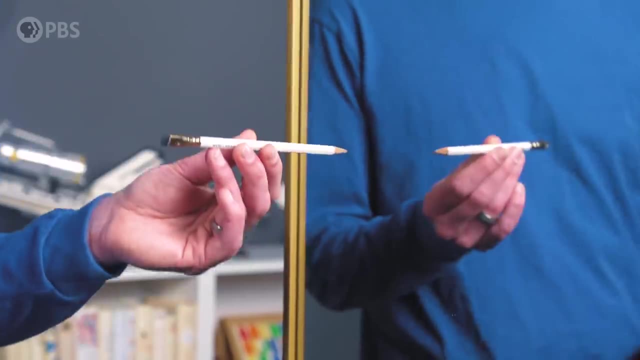 When I face the pencil to the left, well, the mirror pencil is also pointing to the left. If I point it up, then the antipencil is also pointing up. But if I point the pencil into the mirror, well, then the mirror pencil is pointing the. 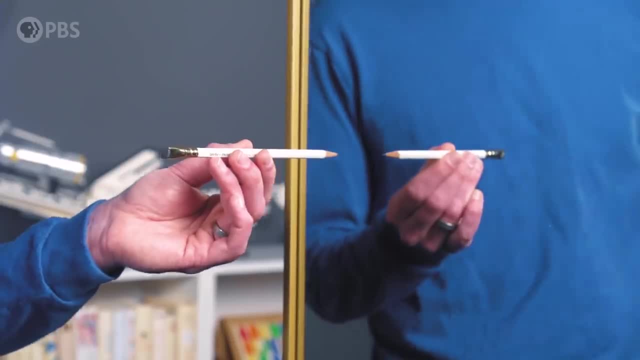 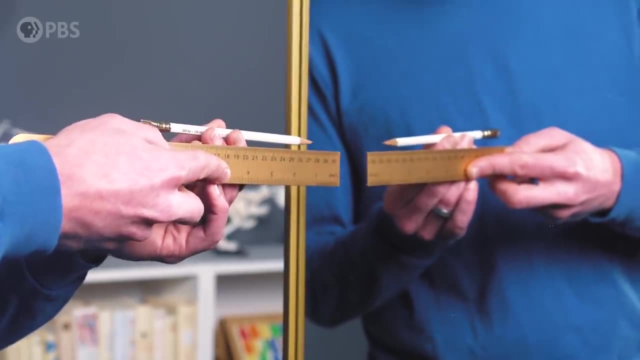 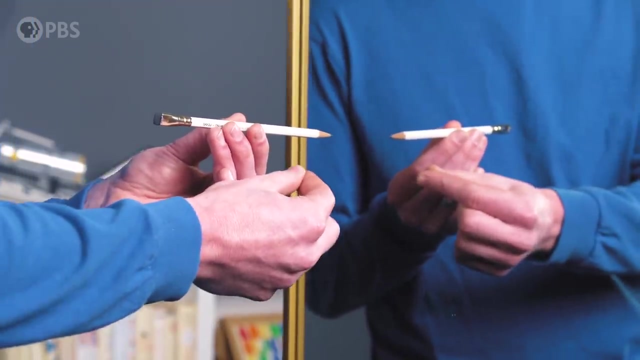 opposite direction. back at me. Watch this. The tip of that pencil is maybe 3 centimeters away from the mirror And the eraser end is maybe 20 centimeters away. The mirror has simply reversed these coordinates along this axis So that the antipencil is pointing to the left. 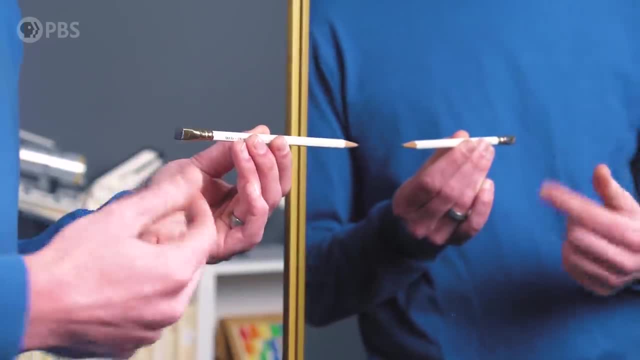 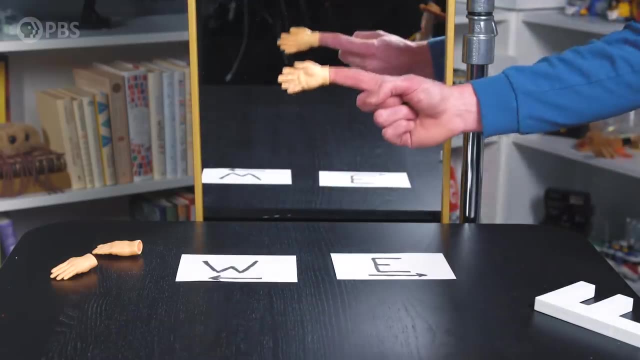 The tip of my tip is minus 3 centimeters and the anti-eraser is minus 20.. Or let's say that this side of the mirror is east and this side is west. When I point west, mirror me points west too. 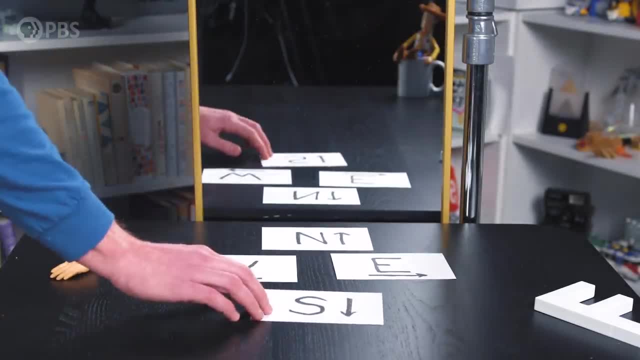 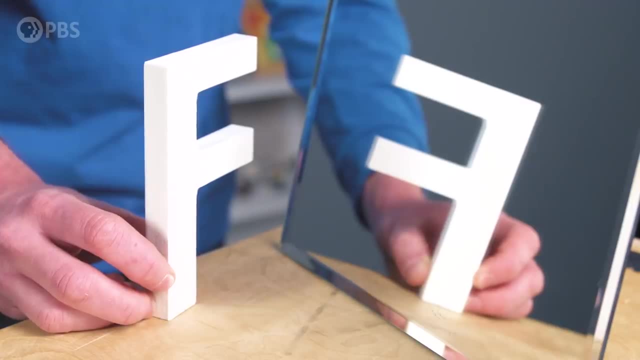 But if say this is north and this is south, when I point north, mirror me points south. But if mirrors flip back to front, then why does text look reversed left to right? Because it's us that's doing the reversing. 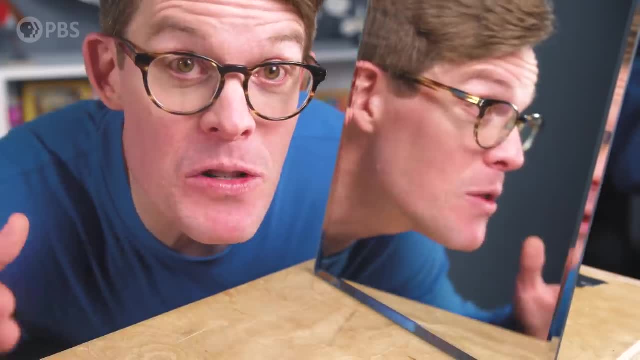 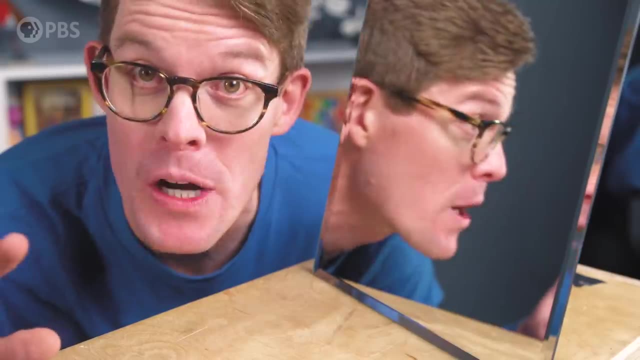 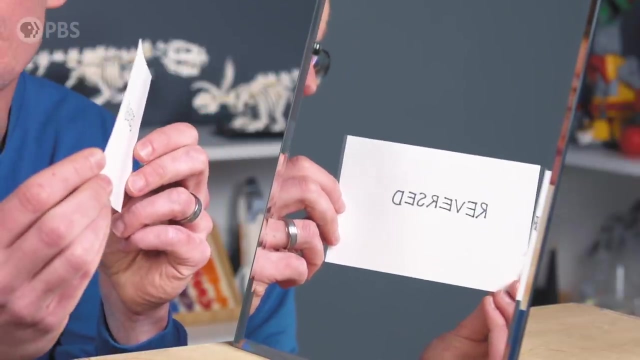 They're just showing us what we show them. See, mirrors don't reverse text at all. You just gotta know how to speak their language. Now that you know how mirrors really work, we can have some fun with them. Now, normally, mirrors make text look reversed because we reverse it. 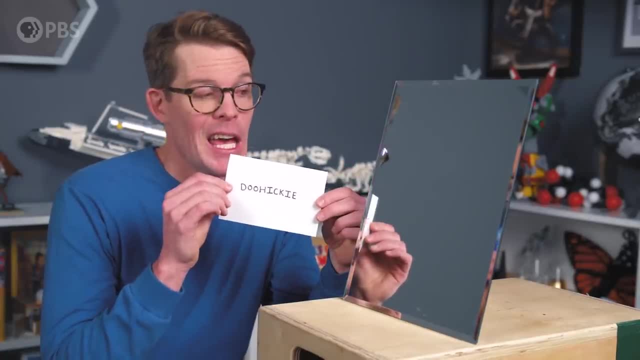 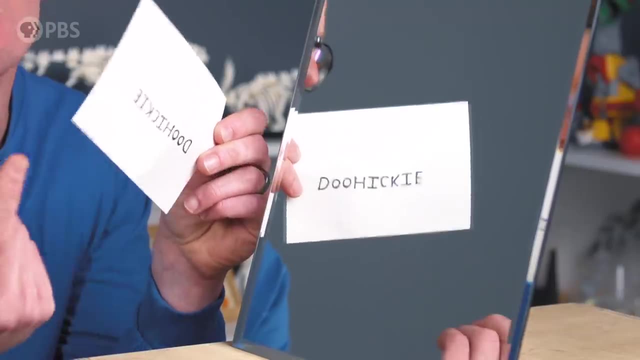 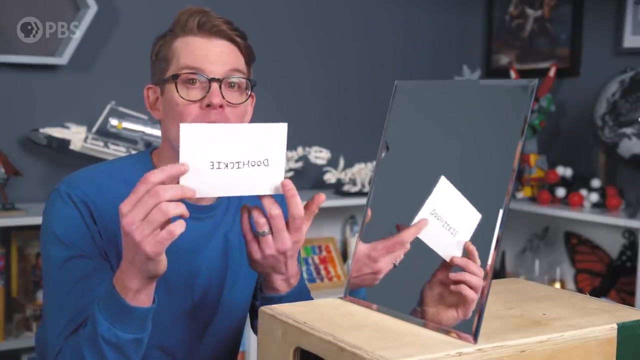 Just as we'd expect, But I happen to have here a doohickey And this prevents this mirror from reversing how it normally would. Of course, that's a trick. I actually showed it to the mirror upside down. Each letter in this word is symmetric along a horizontal axis. 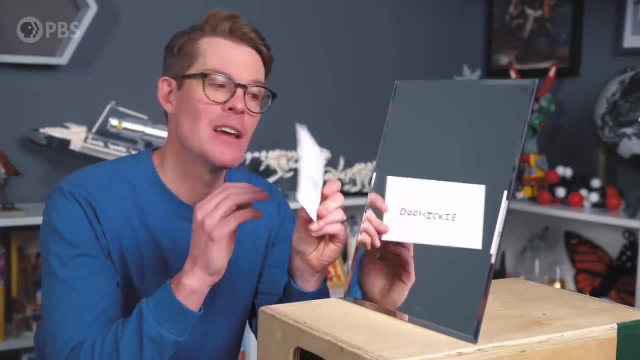 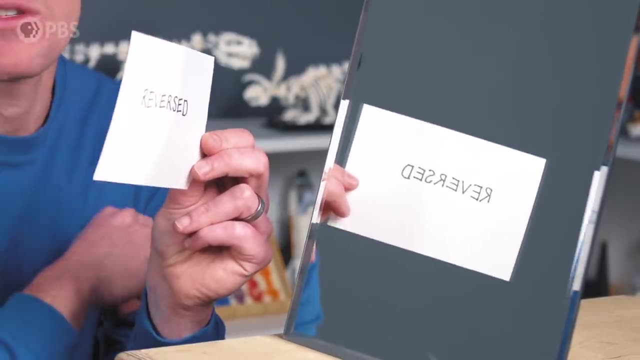 So when I present it to the mirror flipped along that axis, we can read the reflection normally, While this word- because I flipped it along a vertical axis- is reversed. You can even play a trick on your friends by writing out words like these and then: 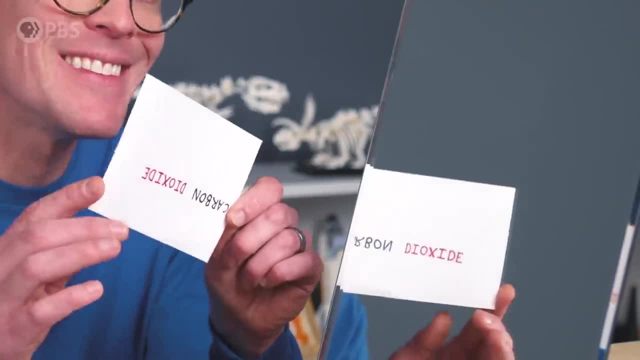 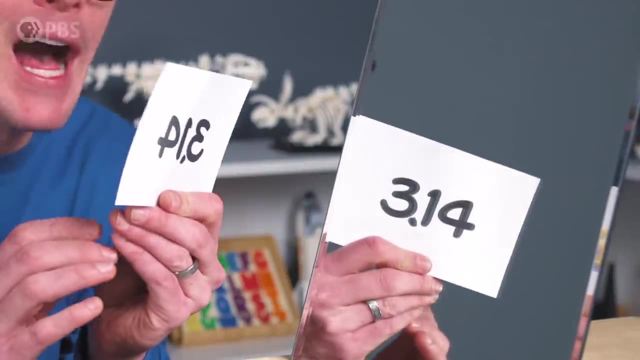 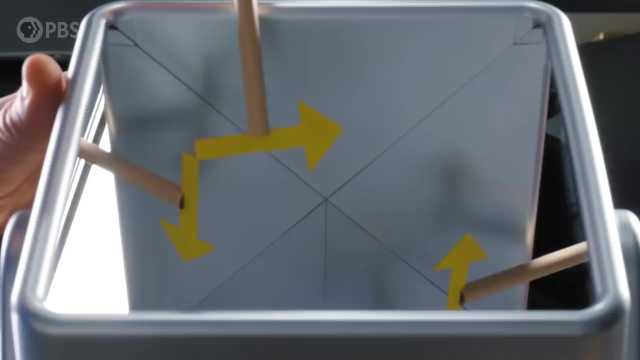 telling them that your magic mirror doesn't reverse red text or that your magic mirror can turn pi into pi. You know that mirror from earlier that didn't reverse images. That's actually two mirrors. They're carefully aligned edge to edge at a right angle. 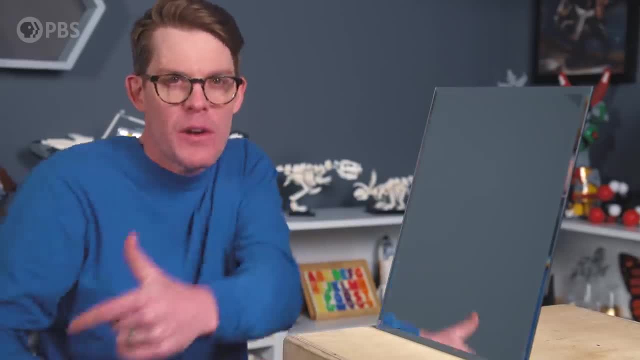 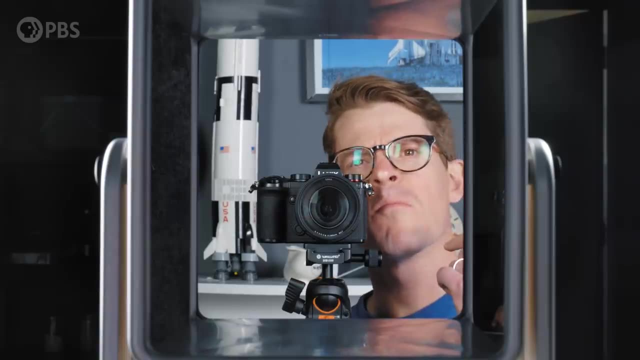 The image is actually reflected back to you twice, reversing the reversal to unreverse it. And yes, in a mirror like this, you see yourself as others actually see you. So why do people say that mirrors reverse left and right when they clearly don't? 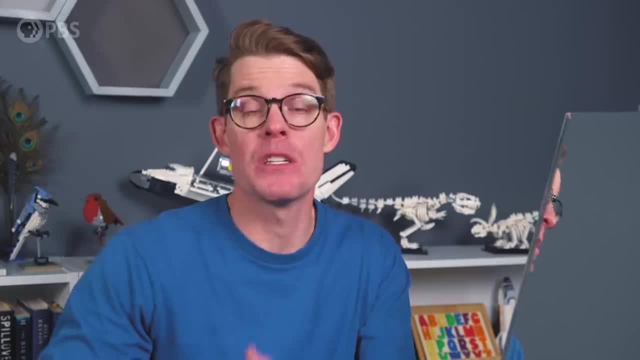 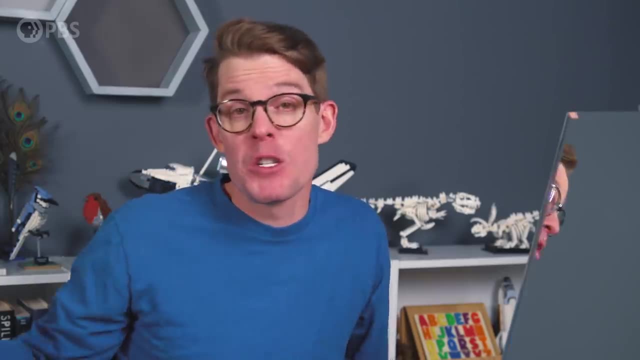 I think it's because they don't see themselves as others. They see themselves as others. I think we just lack the right language to describe what we're seeing, because we rarely put concepts like these into words. I don't know, maybe for four-dimensional people this is very easy. 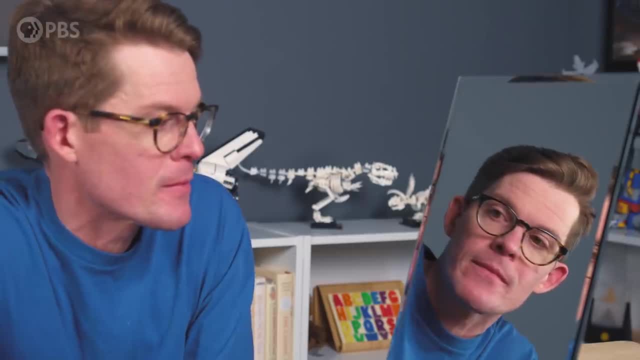 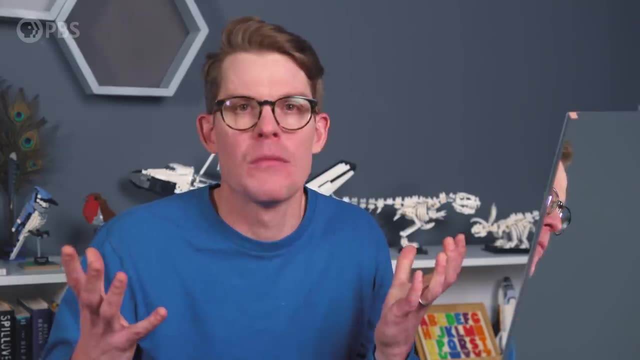 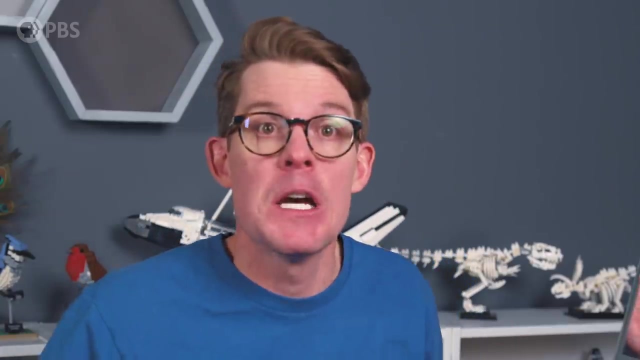 But for us lowly 3D humans, we imagine it's actually us inside the mirror looking back, And since we know what our right and left are, well, we know what their right and left are. So a mirror can teach us interesting lessons about geometry and physics, but they might. 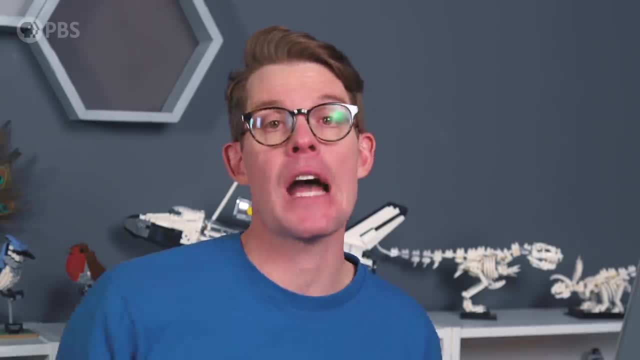 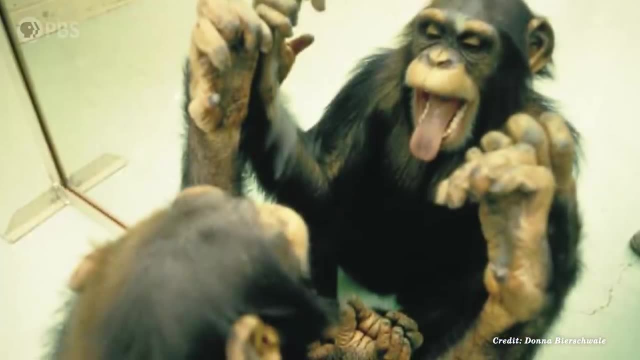 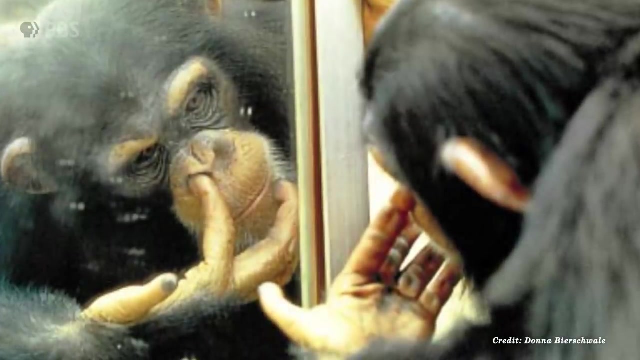 also be able to teach us something about ourselves. An evolutionary psychologist named Gordon Gallup did a famous experiment where he put a mirror in front of some chimpanzees. At first they attacked the reflection. they saw as if it was a stranger, But pretty quickly they started to use the mirror the way we do to look at themselves. 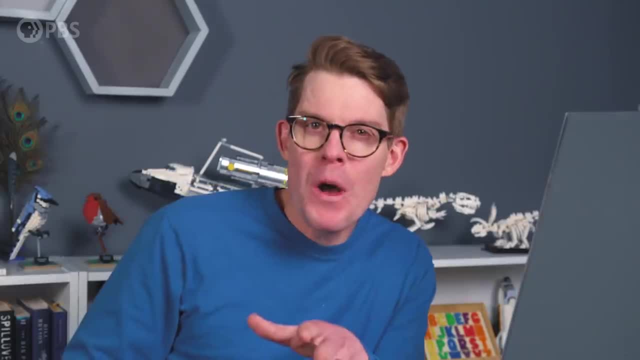 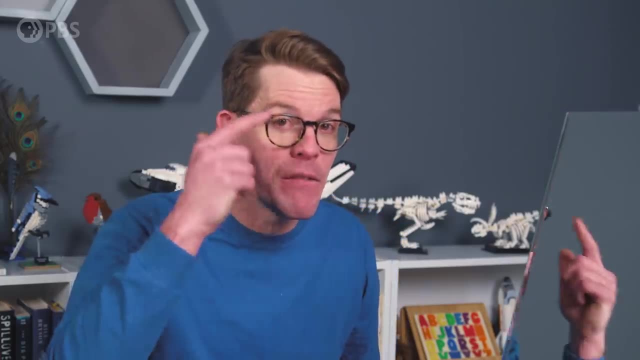 cleaning their teeth, grooming their bodies, but did they know that was them? Well, the chimps were put to sleep temporarily and a red mark was dabbed on their face. When they woke up, they looked at the mirror and they touched their fingers to the paint. 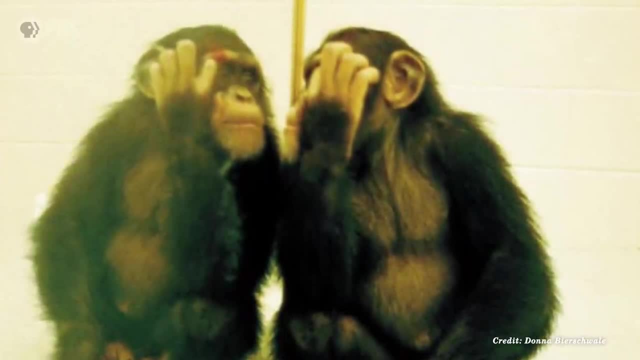 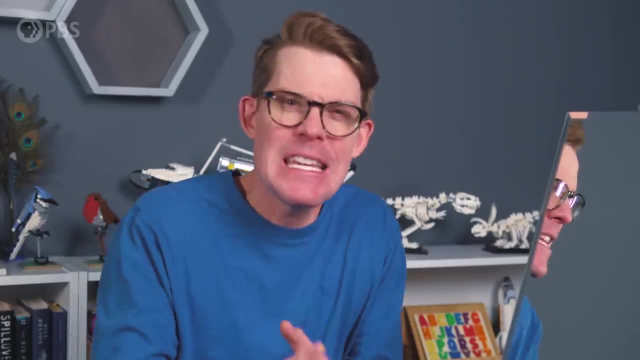 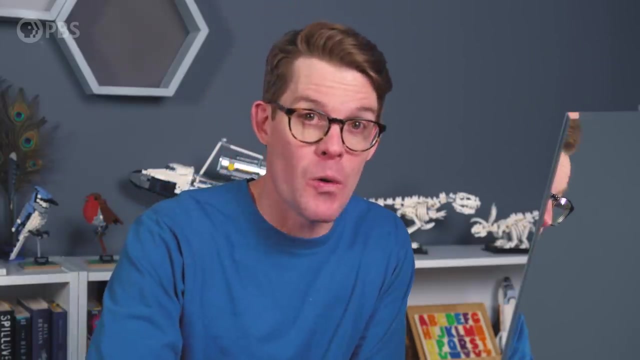 on their faces, not to their reflections. Along with bonobos, orangutans and a few other species, there's only a handful of animals that recognize that what they see in the mirror is themselves. Any species that can recognize itself in a mirror not only has a mind of its own, but 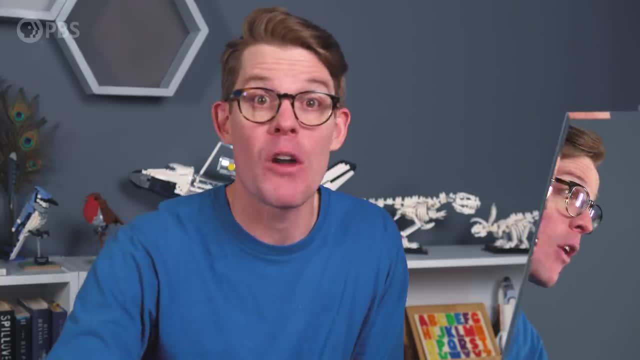 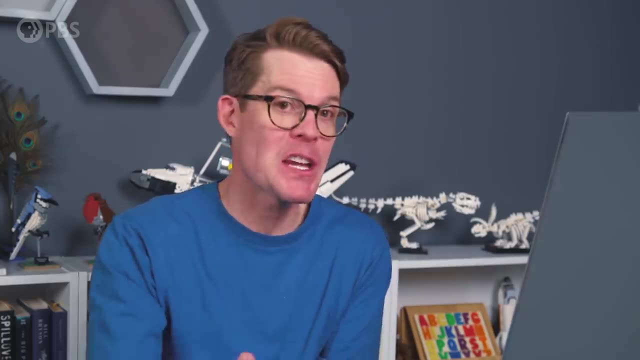 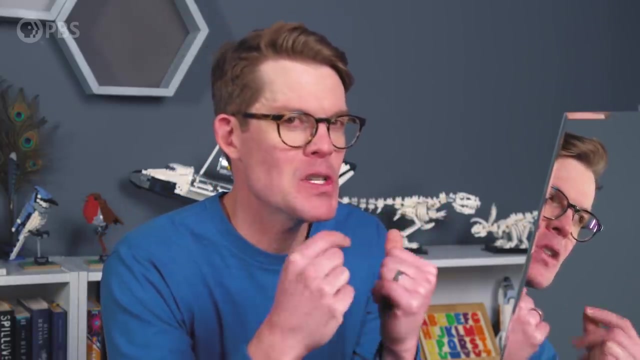 also has the potential to recognize that other creatures have their own minds. 3. They express empathy and complex emotions like that. But humans are special among this group because we not only realize that what we see in the mirror is us, but also that it's not exactly us. 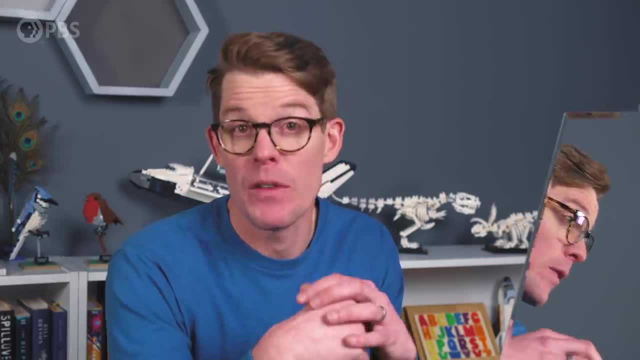 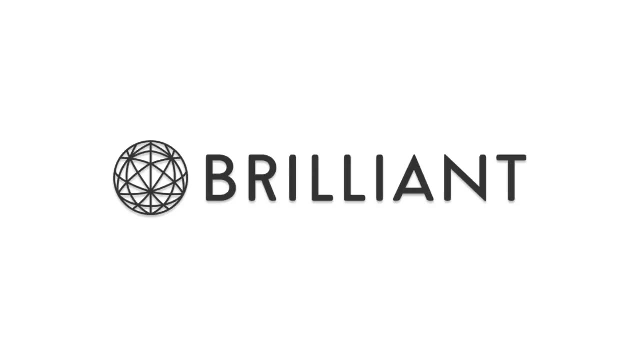 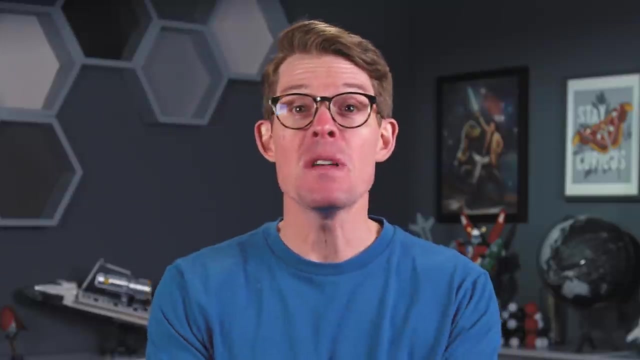 Plus, I'd like to see a chimpanzee make this video. Stay curious, And thank you to Brilliant for supporting PBS. Brilliant is an online learning platform for STEM With hands-on interactive lessons. This platform is for curious learners, both young and old, professional and inexperienced. 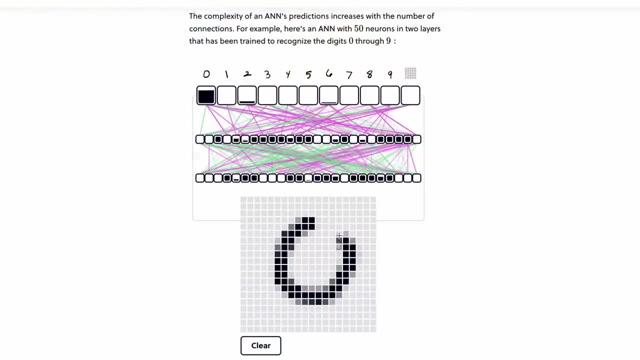 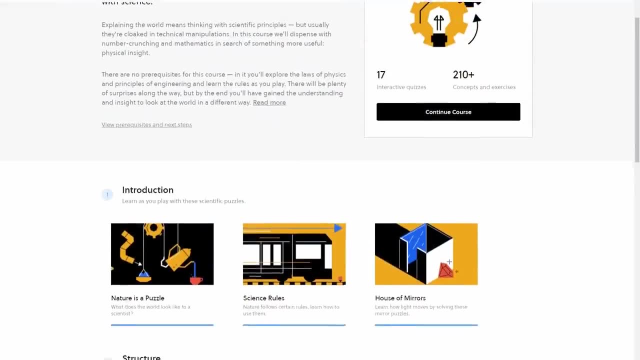 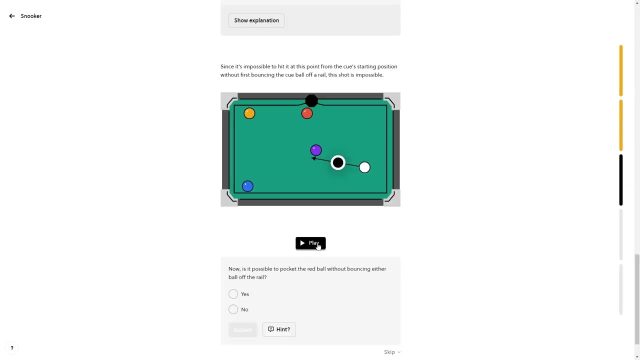 You'll get to see science in a new way through visual examples. For example, for those who want to strengthen their physics knowledge, you can begin Brilliant's scientific thinking course, where you can explore the laws of physics and the principles of engineering and the rules that make them work, while solving puzzles.